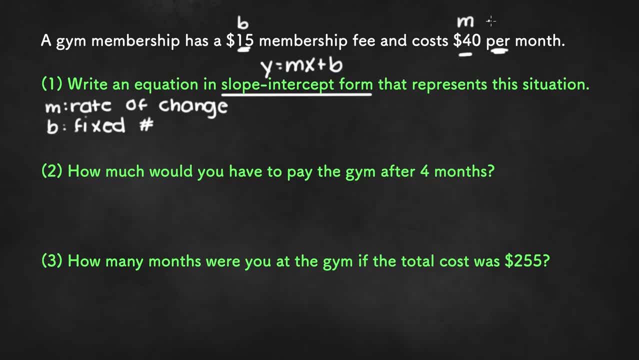 we can assume that this $40, we can assume that this $40, this $40 is m. So once we plug that into the equation, we get y equals 40x plus 15.. And that'll be the answer to the first part. 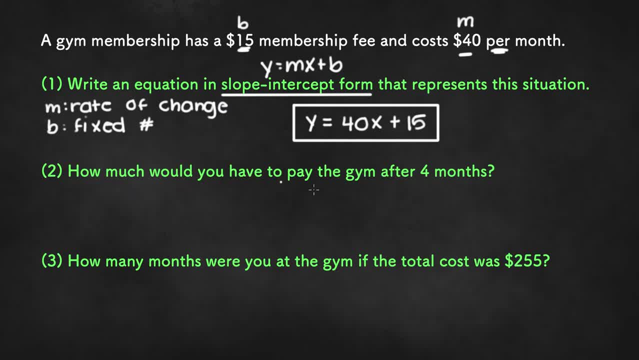 Now the next part asks how much would you have to pay the gym after four months? So before we work on this question, let's define x and y in terms of the word problem given here. So, first of all, y is the total. 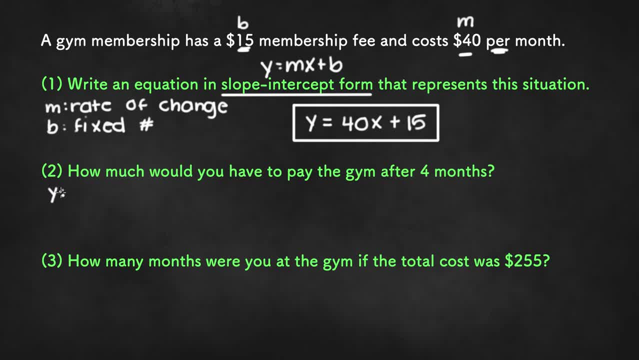 And in this case, since we are talking about money, y would be the total cost And x is related to the m value, Since m is 40 and the word problem says $40 per month, x is the number of months. So we are asked to find the total cost of the gym. 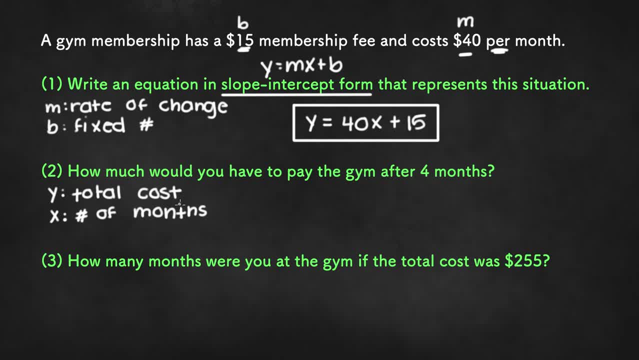 after four months. That means we are finding y when x equals 4.. So let's plug in 4 for x in the equation and solve to get our y value. So if we plug it in, we get y equals 40 times 4 plus 15.. 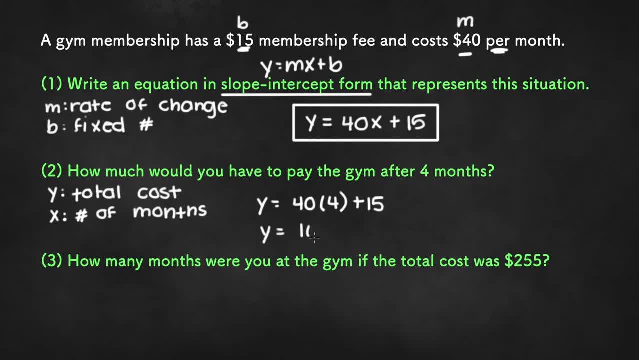 So 40 times 4 is 40.. 40 times 4 is 160.. And 160 plus 15 is 175.. So you would have to pay the gym $175 if you were a member for four months. So the last part of this word problem asks: 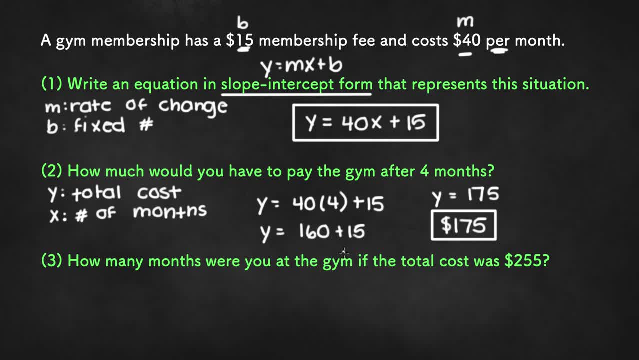 how many months were you at the gym if the total cost was $255?? Since we are given the total cost or the y value and we are asked to find the number of months, we need to plug in 255 for y and solve for x.